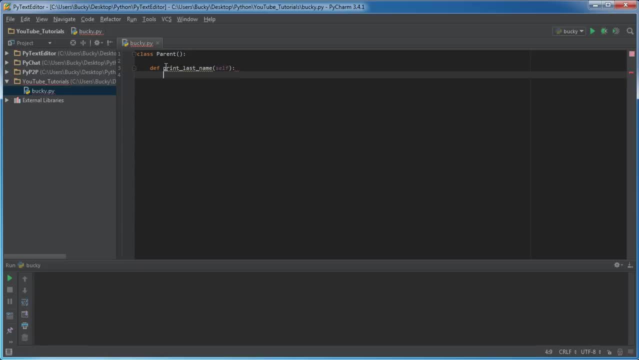 last name. So of course, this just looks like a normal class right now. And my parents last name is the same of mine, of course, so Roberts. So right now, this parent doesn't have any cool land, doesn't have a million dollars to leave me. all it has this is lonely old function. So I'm going to make another class right here and I'm going to name it child And, just like before, we can start building functions. But check this out. 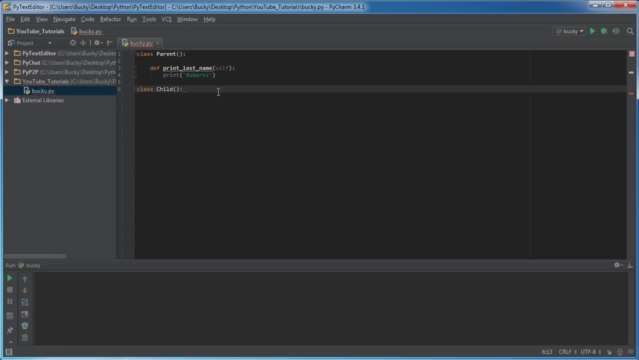 If you're wondering: why do you have these empty parentheses right here? Well, inside these parentheses, what you can pretty much type is the name of a class that you want to inherit from. So whenever I typed parent inside here, what I'm telling Python is: okay, look for a parent class, get everything inside that class And right now it's pretty boring- just one function and pretty much pass it on to your child. 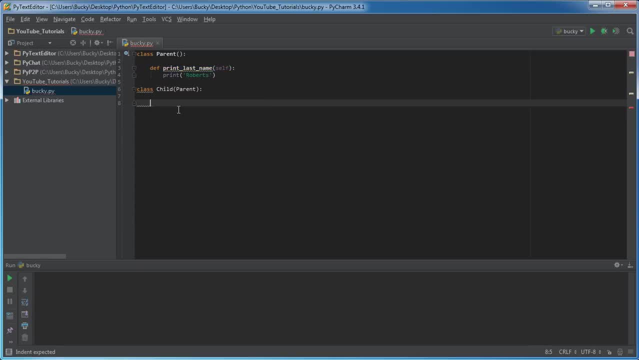 So right now, even though it looks like this child class is empty, it actually has- in other words, it actually just inherited this print last name function. So let's go ahead and make one normal function in the child class. I'll go print first name And this will just be. it'll just be a normal function that belongs to the child And it'll just print out my first name, which is Bucky. 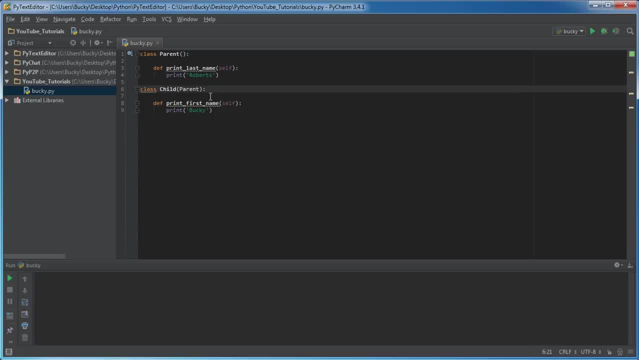 So check this out. Right now it looks like there's one function in parent and one function in child, But that's not actually how Python sees it. Well, Python sees is this one function parent, And since this child inherited everything from the parent, it actually has print last name and print first name. Don't believe me- I wouldn't either, because I lie about stuff a lot, But in this case I am telling the truth. 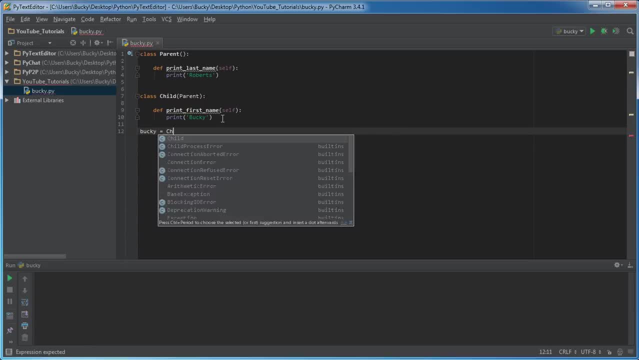 So I'll make a function or, excuse me, an object called Bucky And it's going to belong to that child class. Now check this out: If I put Bucky- come on you stupid frickin carpal tunnel glove- I can do print first name And we already know that because the functions right in that class. But did you know I can also do print last name and check this out. 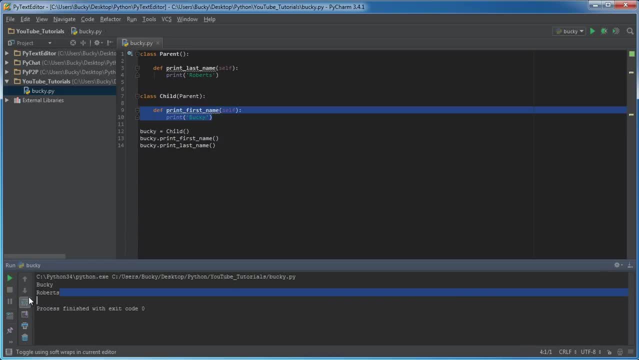 I'm going to print Bucky, which is just a normal function, And also Roberts, which is a function that it inherited from the parent. So that's the basics, the very basics of inheritance. Pretty much saying, okay, what class do you want to get stuff from? So pretty much doesn't literally do this, but goes that class, copies everything and paste it right in child. Simple enough, Guys understand it Good. 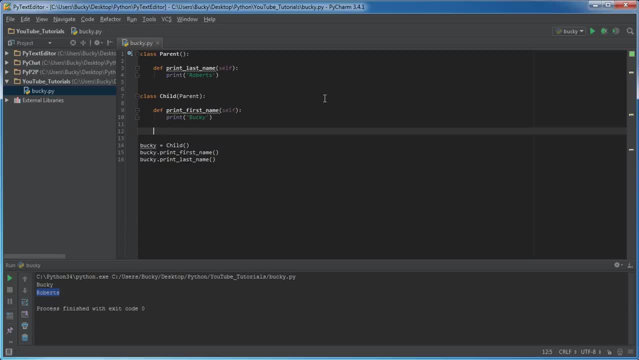 So now we're going to talk to you guys about something that's a little bit more advanced, a little bit more confusing. So right now we have print last name, basically as a child function that it inherited. Now what we can also do is we can also have the option of overriding- Overriding- Wow, that's for some reason hard for me to say. The child can override that function. So what we can do is this: 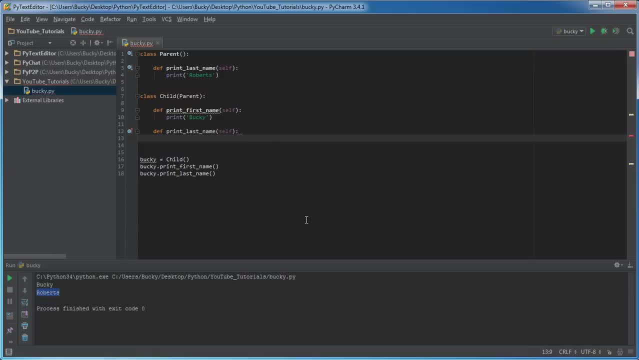 We can print last name And also I'll just, like I don't know, make this print something called Schnitzelberg. So I got to tell you guys a story real quick, because I don't have a therapist and I've been meaning to tell someone this for a long time to get it off my chest. But basically, whenever my parents had me, they put Roberts on the birth certificate And that was my last name for a while. 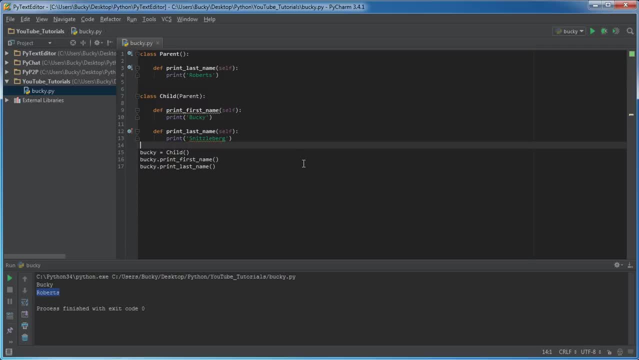 Growing up, Bucky Roberts, Bucky Roberts. in high school, However, I found out that my mom was actually a monkey and I was embarrassed about it, So I ran away from home, I joined the circus and I changed my last name to Schnitzelberg. So, even though I inherited the name Roberts later on in life, I decided to override it to Schnitzelberg. So this is also an option in Python. So check this out.